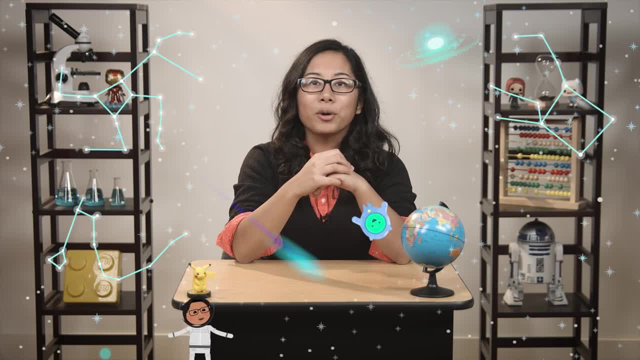 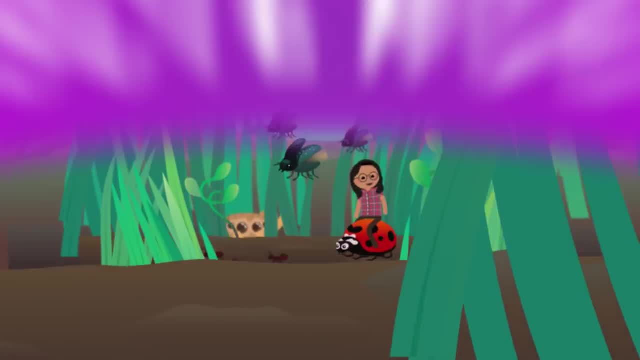 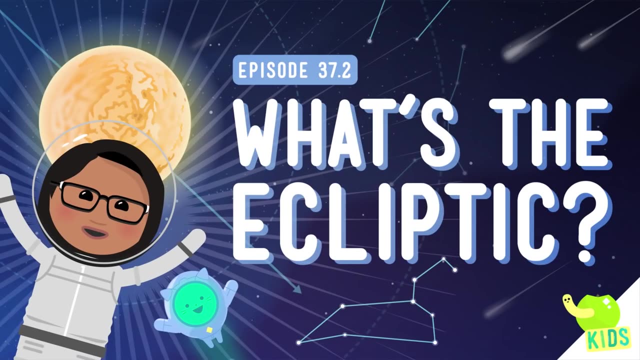 Hello, fellow stargazers. Welcome back to another episode of Tiny Sabrina in Space, also known as Crash Course Kids. I've still got my eye on the sky, particularly those 13 constellations in the zodiac that we learned about earlier. 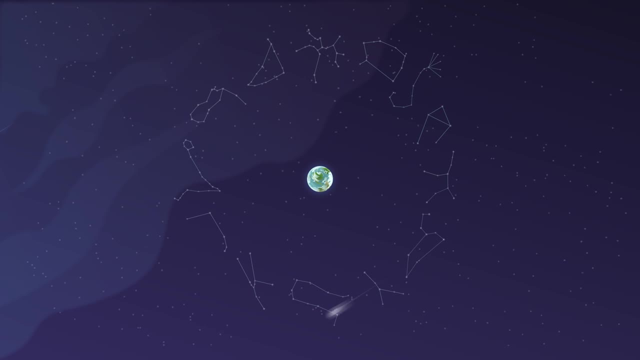 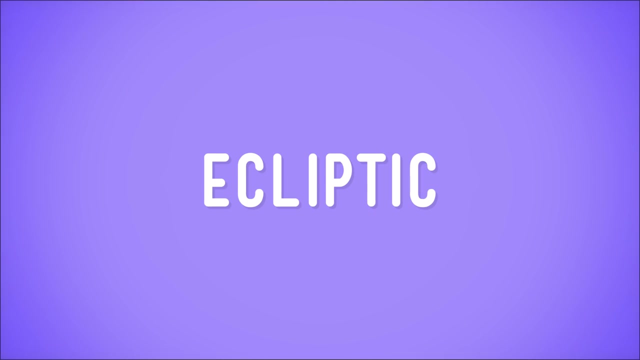 We found out that the zodiac constellations follow a circular path around our planet. Today, we're going to learn more about where our sun falls in this path. I'll give you a hint: It involves something called the ecliptic. 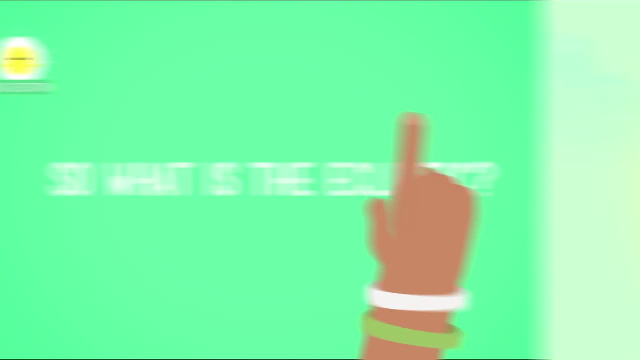 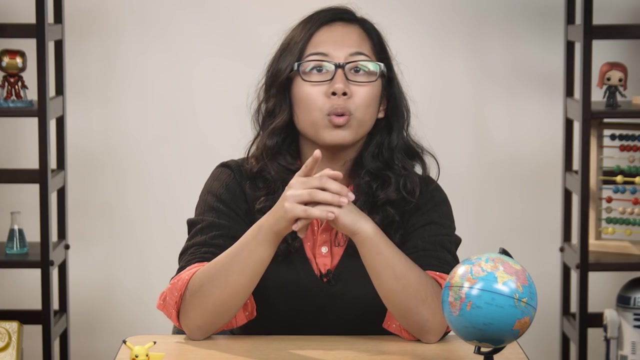 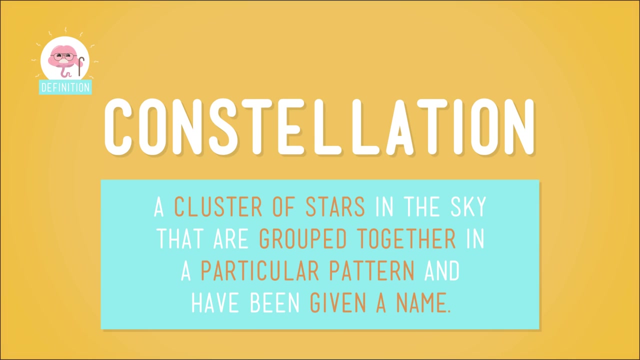 Intriguing. So what is the ecliptic? Before we head into imaginary space to find out, it's time for a quick, well, crash course on astronomy. You know what a constellation is? a cluster of stars in the sky that are grouped together in a particular pattern and have been given a name. 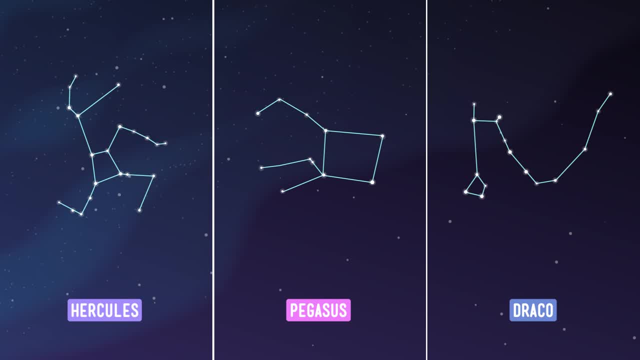 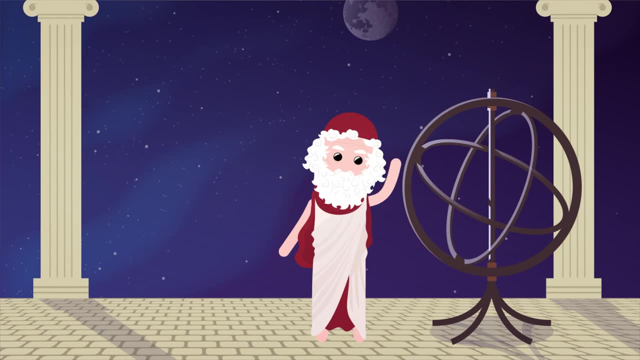 Some of the constellations we've visited so far include Hercules, Pegasus and Draco, And last time we met a group of constellations that form something called the zodiac 13- constellations that have been studied and tracked since ancient times. 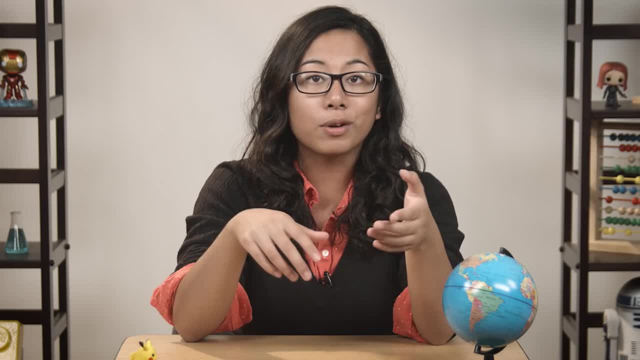 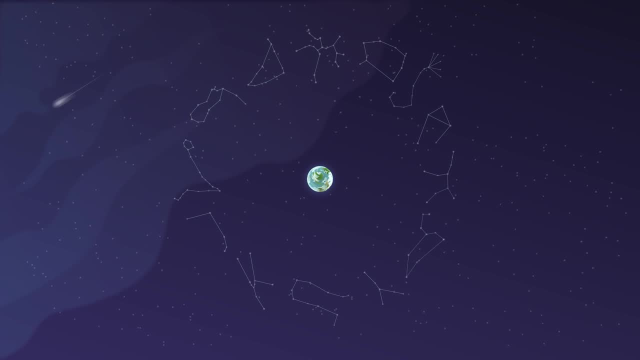 The constellations in the zodiac are all highly visible from Earth during different months of the year, starting with Sagittarius in January and ending with Ophiuchus, And last time we saw how these constellations form a sort of belt-like shape around the Earth. 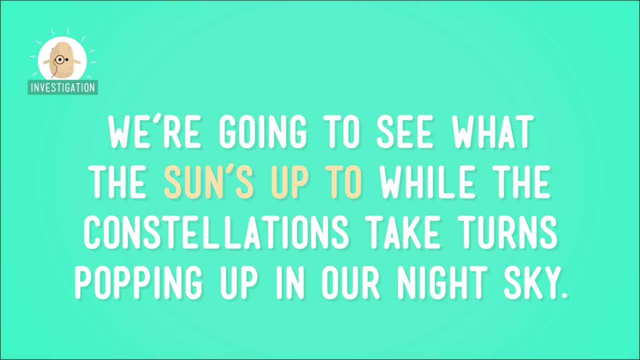 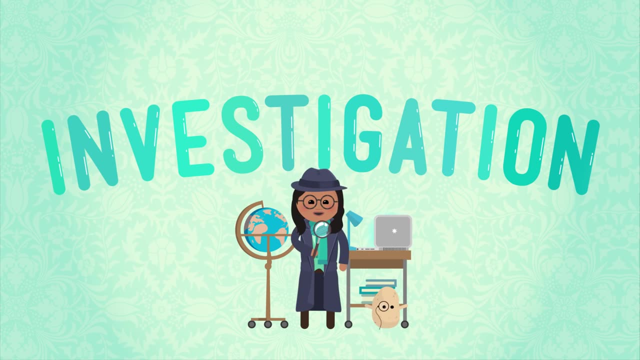 Well, this time we're going to see what the sun's up to while the constellations take turns popping up in our night sky. Okay, so there's Earth in the middle of space, Looking good home planet, And here are the zodiac constellations that surround Earth. 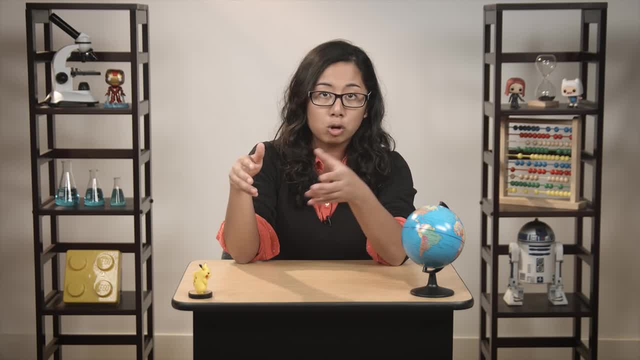 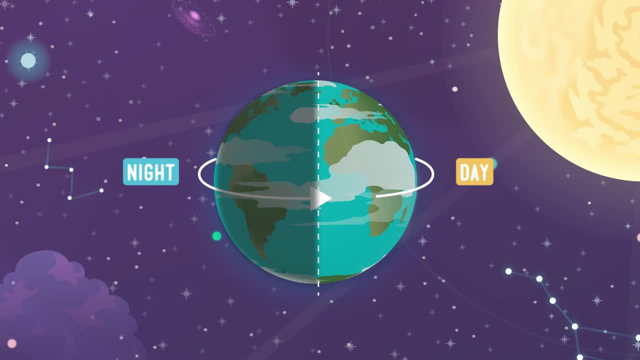 But we've got to make room for another major player in space. You remember the sun, of course. Earth scooch over Sun. head to center stage. You're on. Okay, you already know that Earth rotates on its axis, making a complete turn in one day. 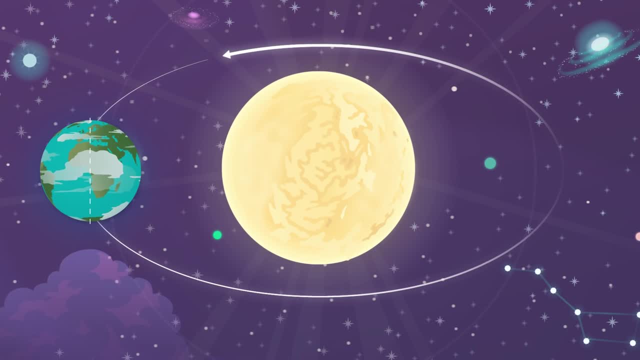 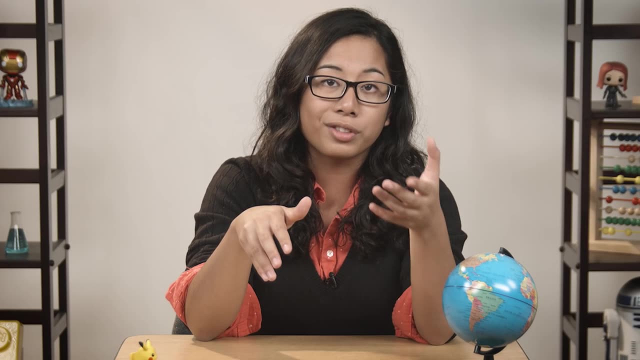 While it's rotating, it also revolves around the sun making one full trip around the sun, And the sun is moving through the stars every year. This movement of the Earth also makes it seem as if the sun is moving through the stars over the course of the year.